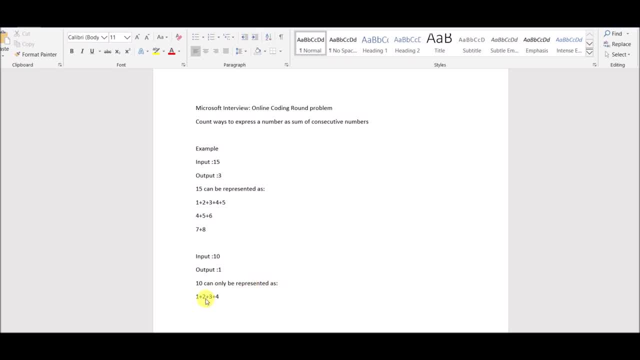 output is only 1 because 10 can be represented as sum of consecutive numbers by only one way: 1 plus 2 plus 3 plus 4. so how to do it? nice, it is the perfect example of how companies can trick you, since it does not require any. 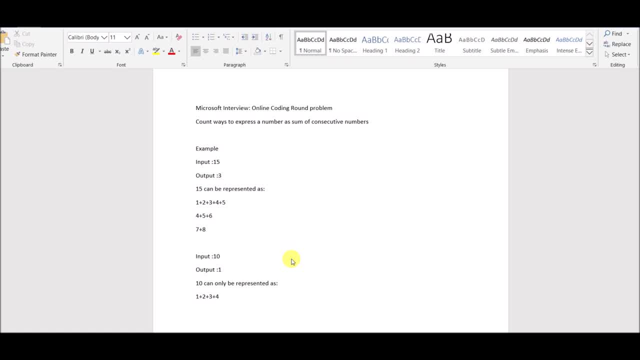 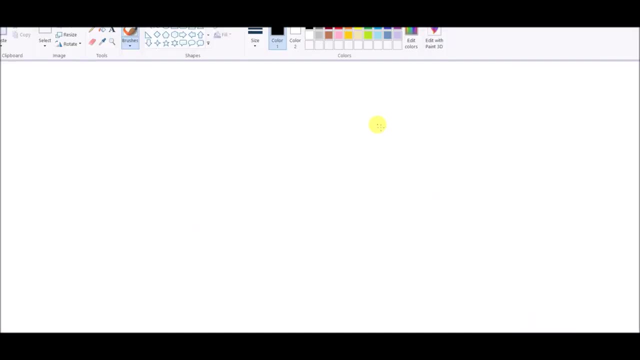 data structure. so it's just a simple problem, but you need to think of it, and this is the first example of how companies can trick you. so, if you are mostly happy with what you are getting out of this step, let's try to compare it with managing an output based on power. so this is the first example of how. 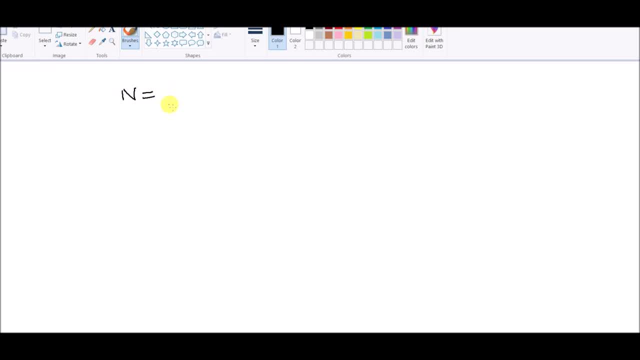 you can kind of run the notion of managing an output based on a given function which is 0, undoing output, instead of building an output based on output is the Heven story. this is the first example of how you can arrange an output based on a given function because you, just you, can multiply or multiply. 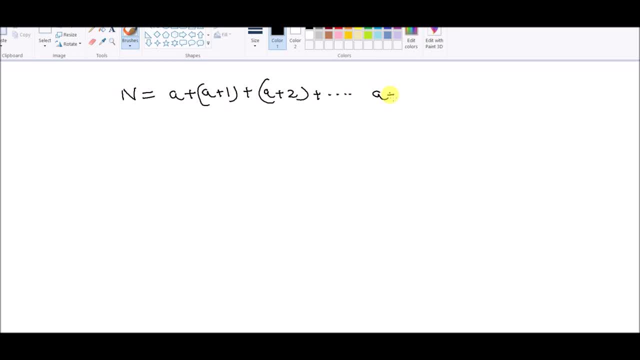 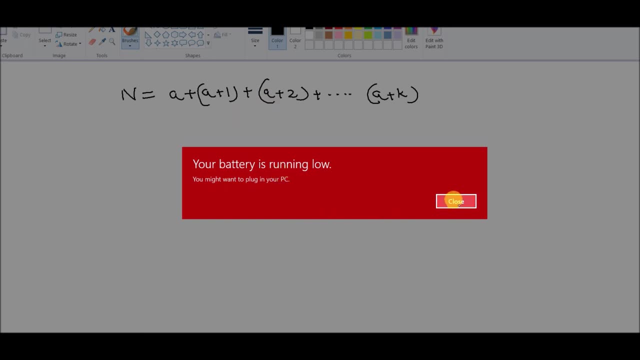 that and denote by that. so you can see that since all the values of each value of a. okay, so i can write number n as this sum of consecutive numbers. if suppose n is a number, then a plus 1 will be the next number, and similarly like that, just a minute. 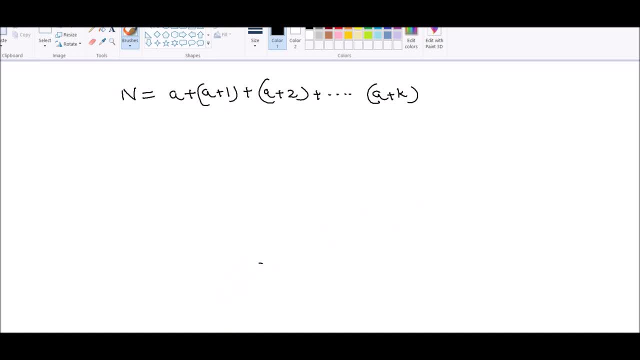 okay, so we can write n as this. this represent consecutive numbers. so now, if you simplify it, so there will be k plus 1 times a. okay, it's uh, 1 plus 2 plus 3, it is k times and this a. so k plus 1 times a. so you can. you can simply write k plus 1 times a, plus 1 plus 2 plus. 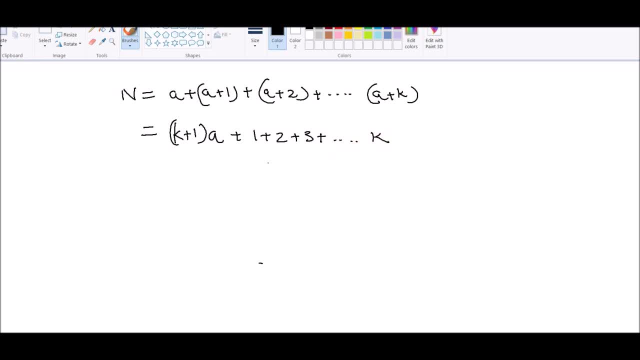 okay, so now this is sum of first natural number and we know the formula. okay, so what? we write k into k plus 1 by 2, sum of first and first k natural numbers. okay, so now this is n. so from this formula we are given n. okay, n is the number. 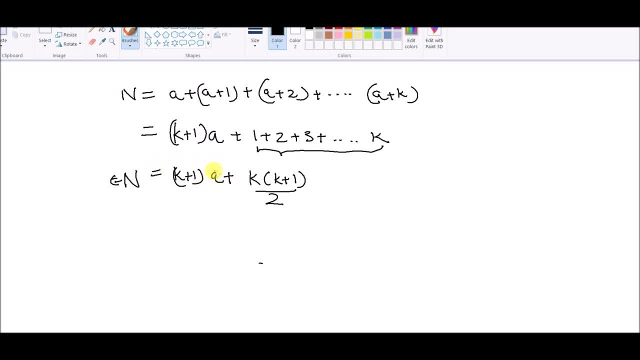 so. so what we need to find? we need to find the a, the first number, okay. so we need to find the value of a. so now it's gonna be n minus, so this is the value of a. okay, for simple mathematics, we are getting this n minus k into k plus 1 by 2 upon k plus 1. 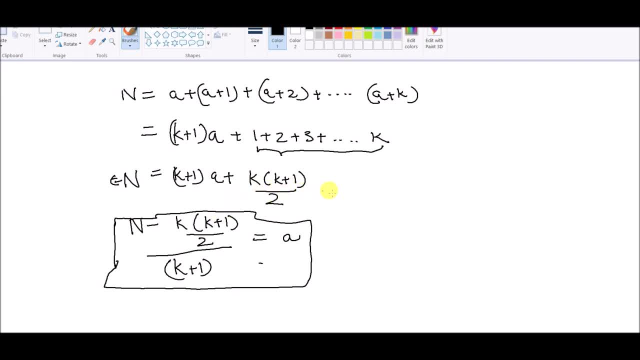 so what we will do? we will just simply, uh, make a loop and we'll increment the value of k and we will check whether we get an integer a or not, if we are getting some integer a, some national number a. so there exists a sum of consecutive numbers and we will simply count. 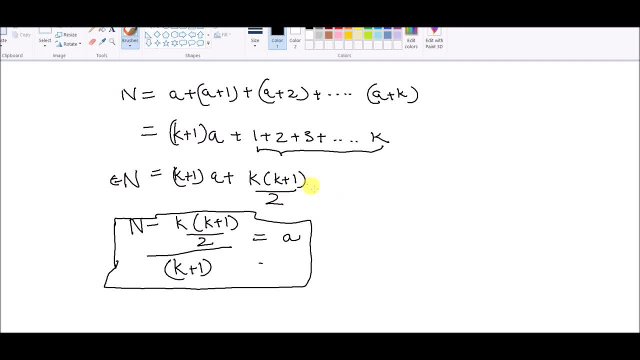 the number of times we are getting a as integer and we'll return it. so it's that simple, k will be the loop variable here, incrementing the value of k. we'll check for every k- okay. for every k less than this, n less than n- okay. so let's jump on to the coding part now. 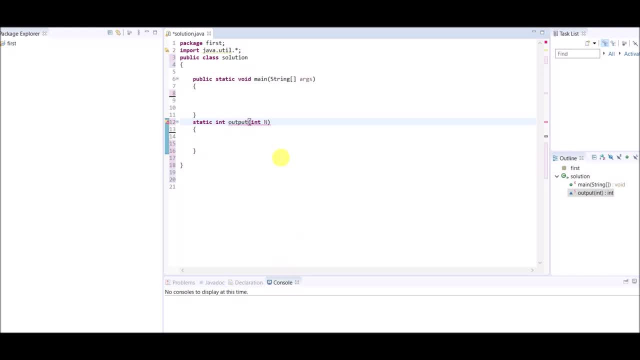 so suppose this is in our platform. i'm doing it in java. okay, so suppose we have this function. okay, output, so that's okay. the return type is in. we'll simply return. uh, the count. okay, just first of all take sound. this will be our answer, okay. 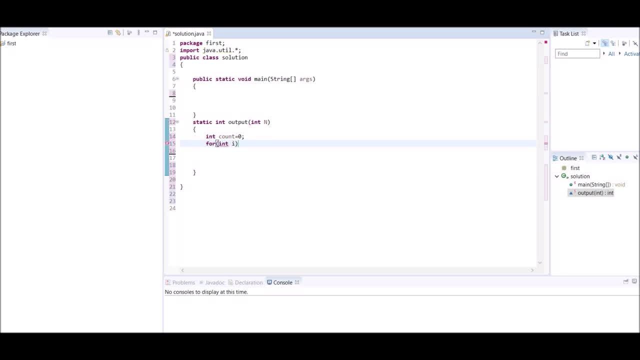 and what do you simply write for loop? uh, the loop variable was k. okay, so k plus 1 and k into okay, so you can see that this. okay, so you can see that this condition came from the equation that we derived in the previous page. okay, so inside which what we will do? we'll simply check whether. 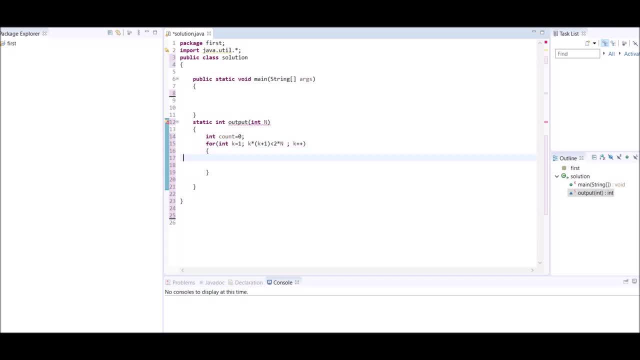 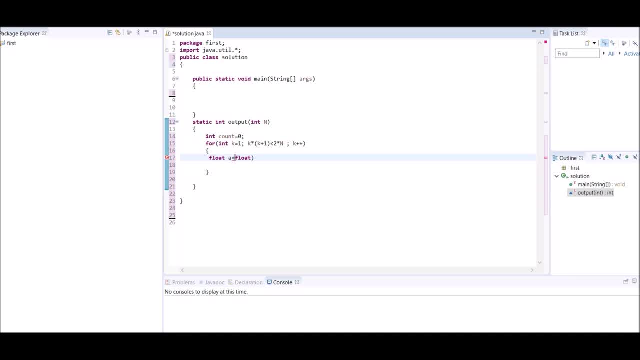 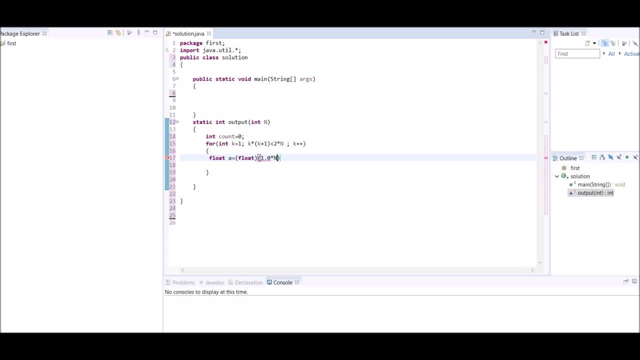 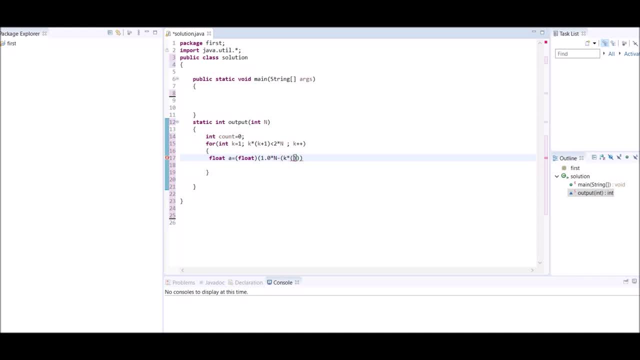 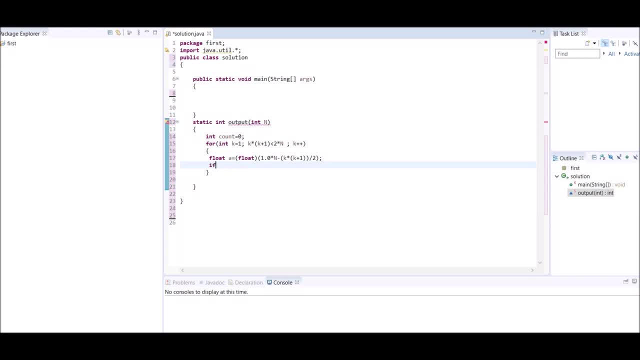 in Java. okay, so we will check whether we are getting a as an integer or not. so simply type cost into and we'll check if we are getting 0.0 or not. so this if statements just simply checks whether the float that we are getting a is an. 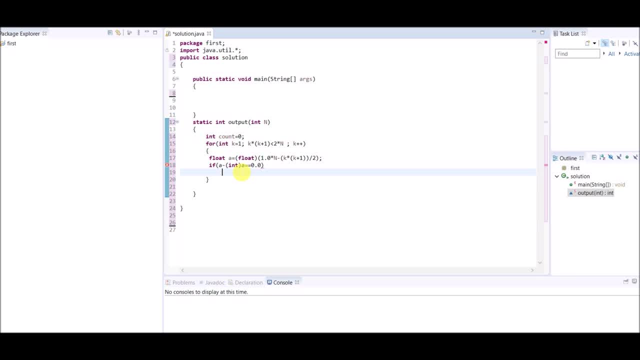 integer or not? well, it is an integer value or not, okay, so the solution only counts just a, then integer, okay, that is it simple, and you will just return count. okay, now from main. mmm, from main you can send the control to here either. I can define it, because what were the test cases?